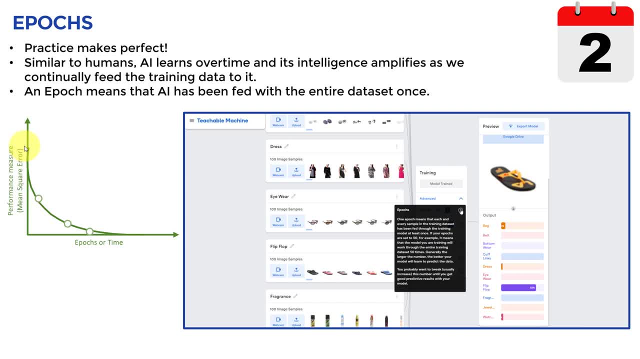 learn from our past expertise, and then we get better over time, and that's why, in general, over time, at epoch 1, you will find that the mean squared error, for example as a metric, tend to go down, And then in epoch 2, the errors tend to go down as well. epoch 3 goes down as well, and over time you will find that the 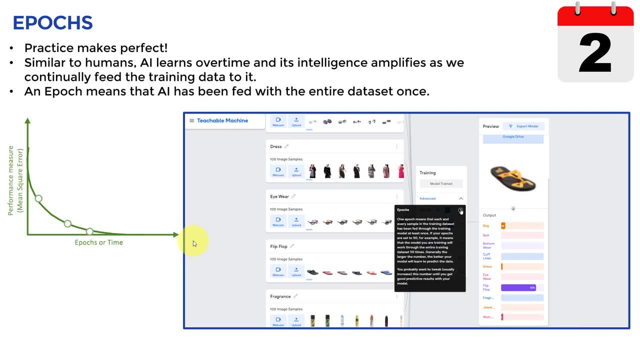 mean squared error, keep going down, and, down and down until we actually stop, and that means the model right now has been trained and is good to be deployed in the field and to actually be exposed to a new data set that it has never seen before during the training phase. okay, so let's go. 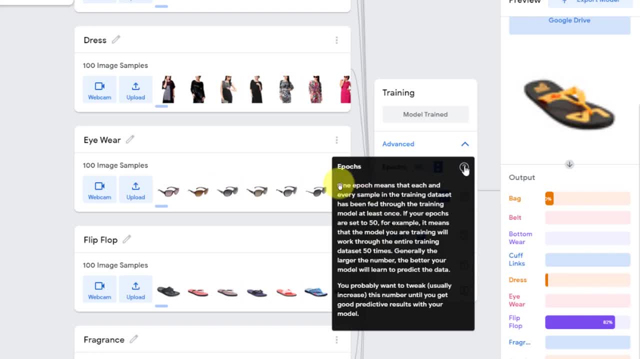 ahead and cover the definition here by google: teachable machines. so one epoch means that each and every sample in the training data set has been fed through the training model at least once. so for example in our case, let's say in the fashion class we had in the original data set, we 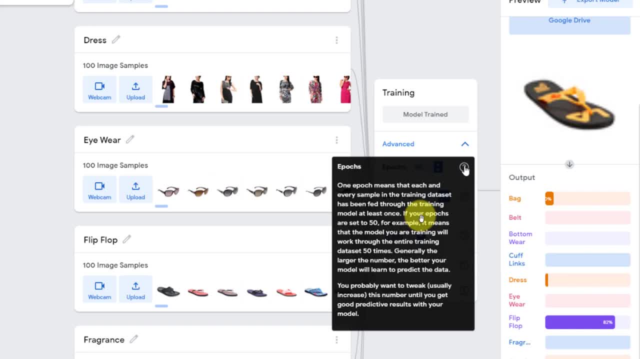 had 10 classes and we had 100 images per class, meaning in total i had thousand images. so if i feed in the thousand images, the entire data set, and i update the weights of the ai model once, that's a good thing. that means now this is an epoch. so if you feed the entire data set, 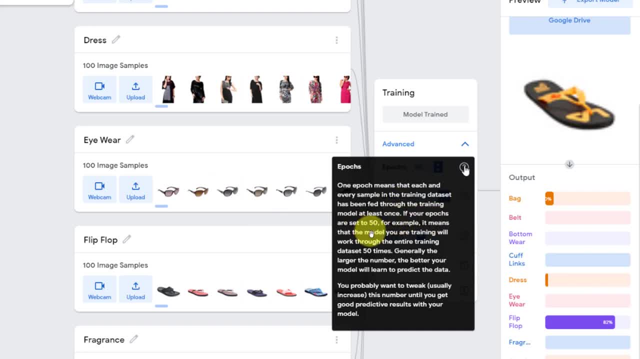 once. that's an epoch. so, for example, if i have, let's say, 50 epochs, that means the model will be exposed to the same data set 50 times. it's like you know, like, like getting the ai model and feeding in the data: please learn that data, learn that data, learn that data. and we're doing it like. 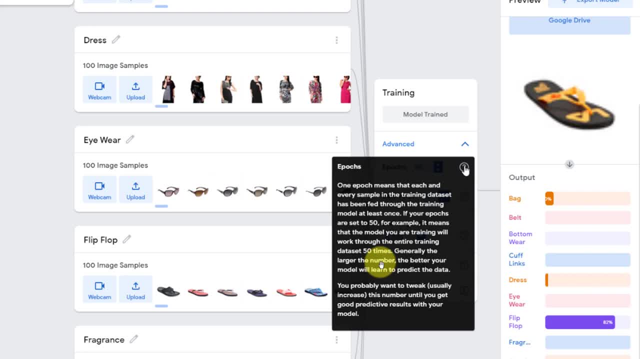 over and over again and that's why it gets better over time, and we do it here. let's say, if we set the epoch to 50, that means we're going to repeat that 50 times and most of the time. if we again increase the number of epochs, you will find that you come up with better predictions over time. 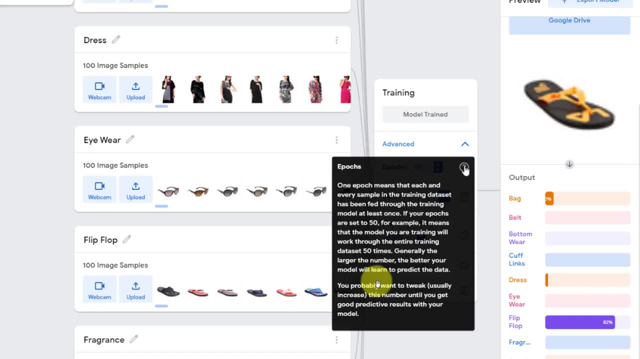 but at some point beyond, let's say, a certain number of course, depending on the complexity of the data, depending on the architecture of the model, you might need not to go, you know, to train it for, let's say, 2000 epochs, and that's why there's a lot of, i would say, human judgment. 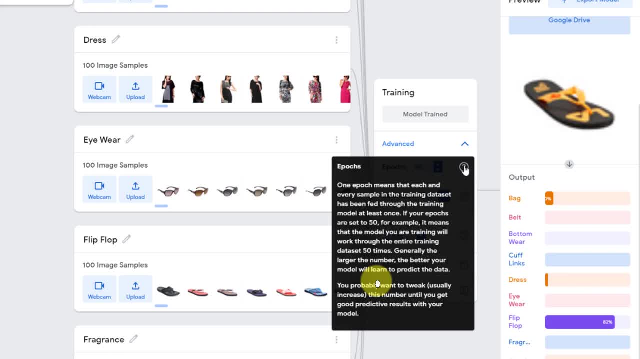 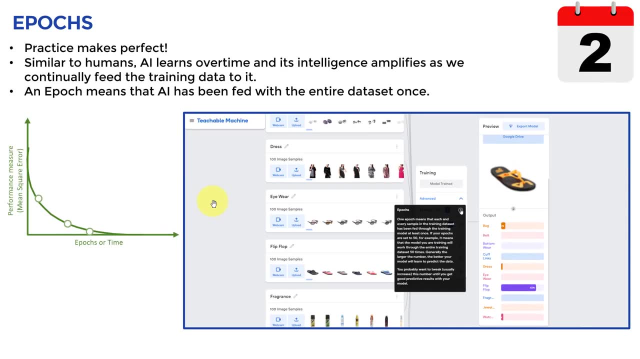 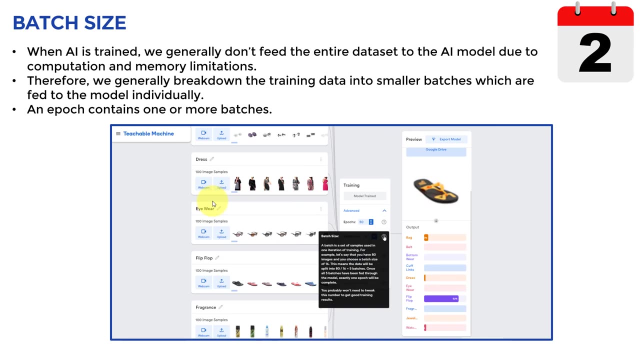 that has to come into play. to get an idea of what would be the best number, google teachable machine set the default value to 50 here. okay, all right, so that covers the first definition. the second definition is known as the batch size. so when ai is trained, we generally don't feed the entire data set to the model in just one shot, and 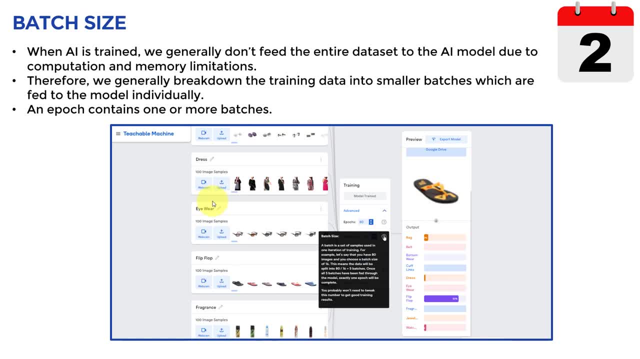 the reason behind it is we might have computation limitation, we might have memory limitation, and that's why, let's say, if we have, for example, thousand images, we don't feed the entire thousand images at once. we break them down into groups or batches, and that's what we're doing here, so we generally break down the entire data. 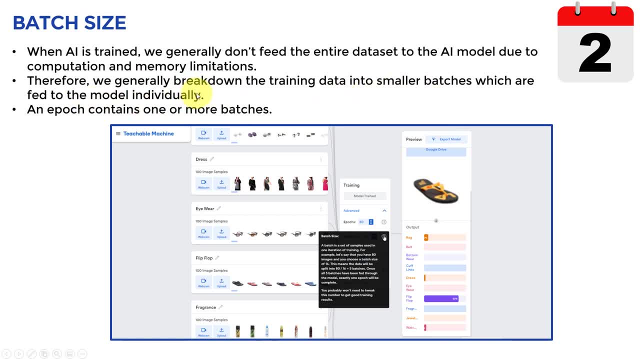 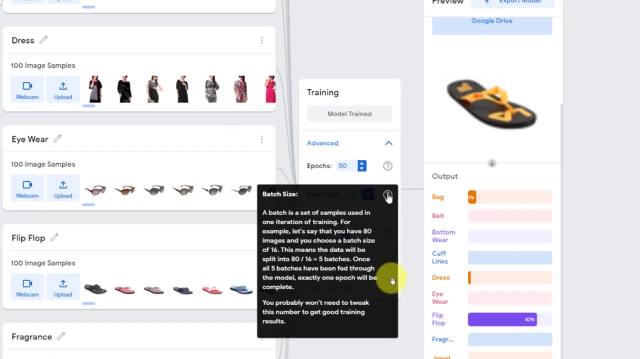 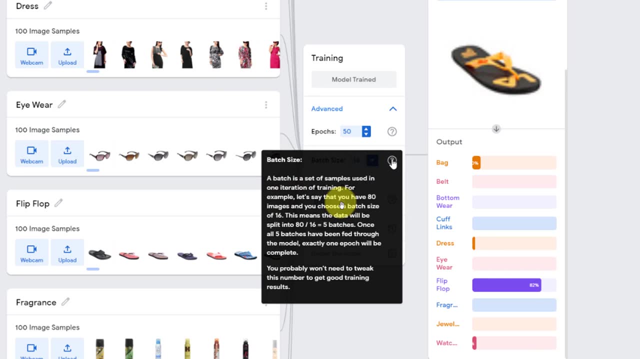 into smaller batches which are fed to the model individually and essentially an epoch. one epoch contains one or more batches. so if you zoom in here, a batch is a set of samples used in one iteration of training. so, for example, if let's assume that i have, let's say, 80 images, for example, and if you choose the batch size to be equals to 16, that means 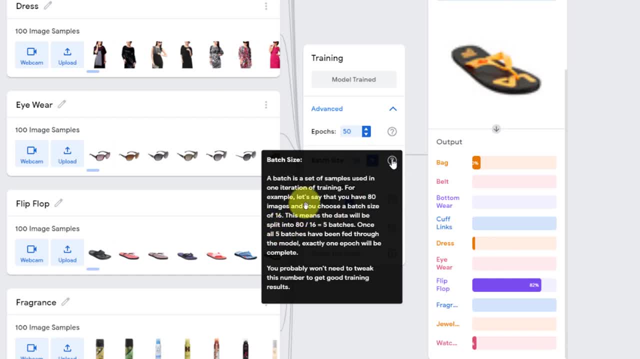 i'm going to take the entire 80 images and i'm going to divide by the batch size, which is 16. i will end up with five batches, meaning i'm going to feed in the data to the model in batches and then we're going to have five of those once all five batches have been fed through the model. 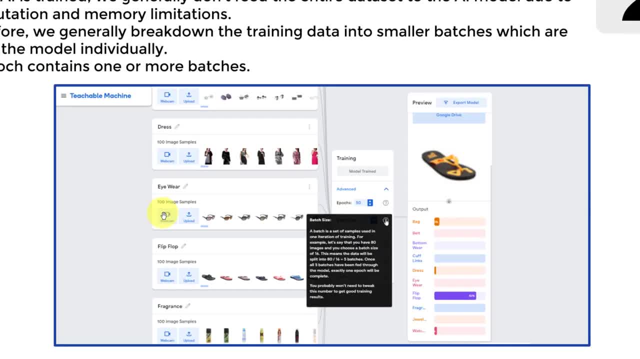 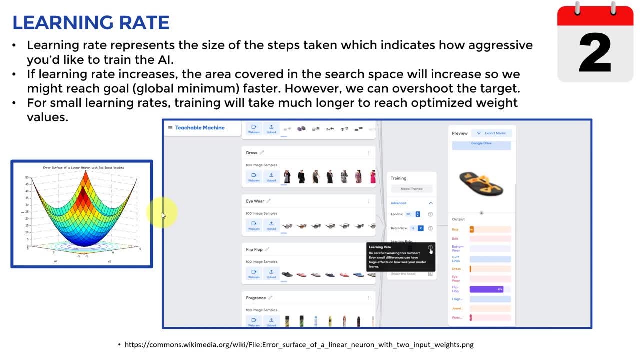 exactly one epoch will be complete. okay, all right, so that simply concludes the second definition. the third definition, which is one of the most important one, is known as the batch size, which is known as the learning rate, and learning rate simply represents the size of the steps taken. 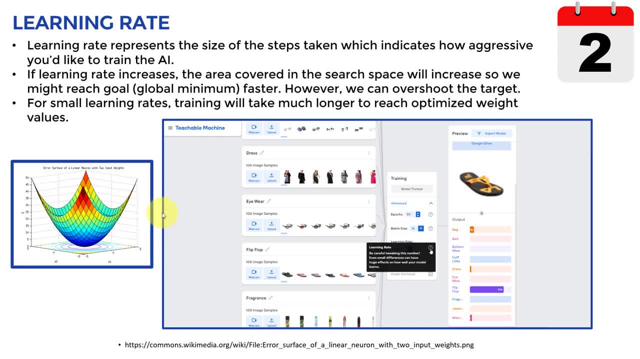 which indicates how aggressive you would like to train the ai model. and think of it this way: let's assume that you are a teacher and you have, let's say a little, for example kid, and you're teaching that kid, for example, how to walk. well, you have two strategies: either to teach that kid, 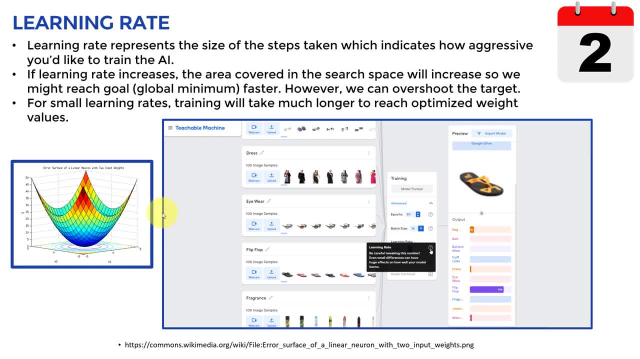 slowly. okay, when i say slowly, that means you are setting the learning rate to be very, very small. or you can just go crazy. you can just set the learning rate to be very, very high and kind of push the boundaries for that kid to actually learn how to walk in a much, much faster. 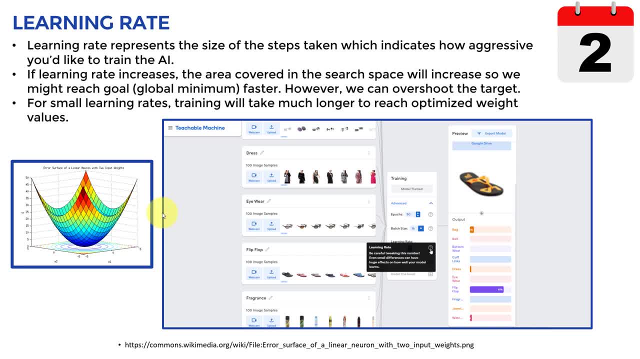 way, and that's pretty much the same idea here. if i increase the learning rate, that means i become really aggressive, meaning i'm going to be training the ai model at a much faster rate, i'm going to be updating the weights a lot more aggressively, and if i set the learning rate to be very, very small, then it's like you know i'm taking 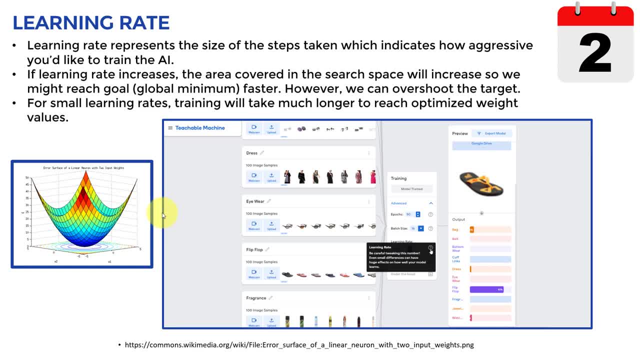 it easy. i'm going to take my time to train the ai model, and that's why, if you set the learning rate to be very small value, then it will take much, much longer time for the ai model to converge. however, if you set the learning rate to be so high, you again you're going to go crazy, right. 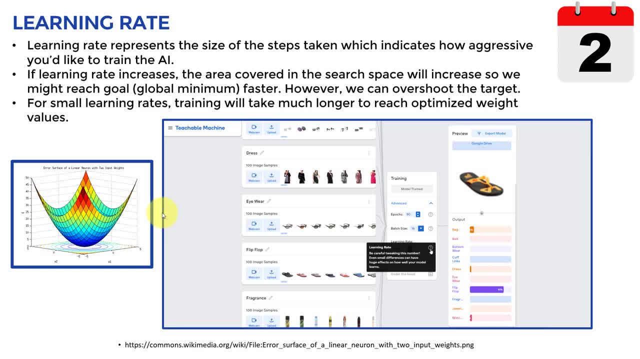 so you're going to be forcing the ai model to converge- what a lot quicker. and the problem is you might reach what we call it. you'll be essentially um over shooting the point that you're looking for. so, for example, what we call a global minimum point. 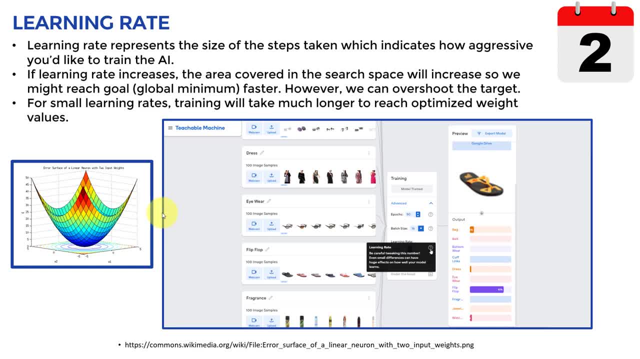 i'm not going to be able to reach it. i'm going to be like shattering across that global minimum, and that's why adjusting the learning rate is an art on its own, and you need to come up with the optimal point- not too small, not too hot, not too large- and that's the overall idea in here. okay, 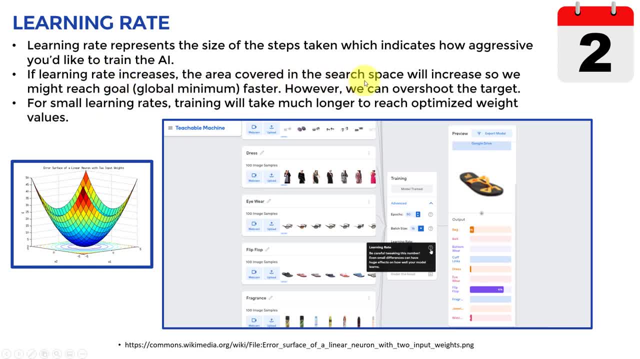 so if the learning rate increases, the area covered in the search space will increase, so we might reach the goal, which is our global minimum, much, much faster. however, we can overshoot the target. so if you guys see here this is essentially the- what we call it, the error surface, and most of the time, what we're trying to do is that we're trying to 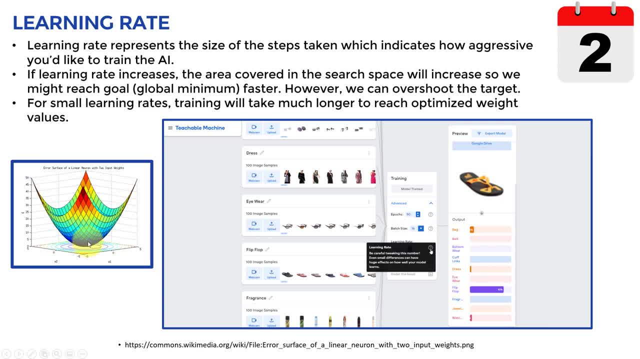 find the point that minimizes the error, like i need to get the minimum error. if you guys remember that we're looking at the error and we're looking at the value of the error and we want to make sure that the error is at least at the minimum value and what we're trying to do is to compare. 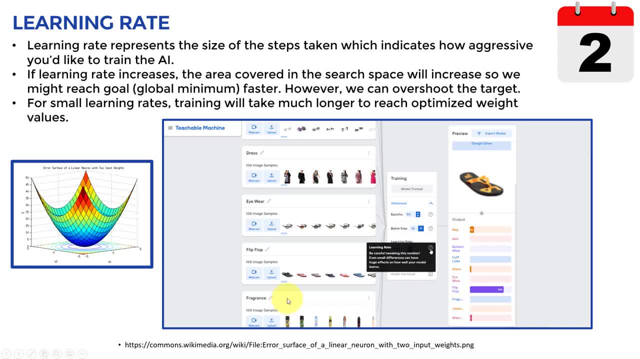 the predictions from the network to the ground truths, to the actual training data, and we calculate the error signal. all what we're looking for is that we're looking for the point where we minimize the error as much as we can. we want to find the minimum error, and that's the overall idea. 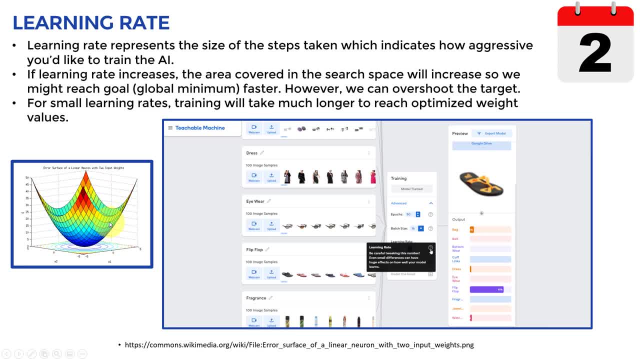 here as well. so if we grab the error surface, this is essentially the point that i'm looking for. that's what i want. so you might achieve that point that you're looking for faster, but the only problem is that you will overshoot that target. however, if you set this, the learning rate to be very small. 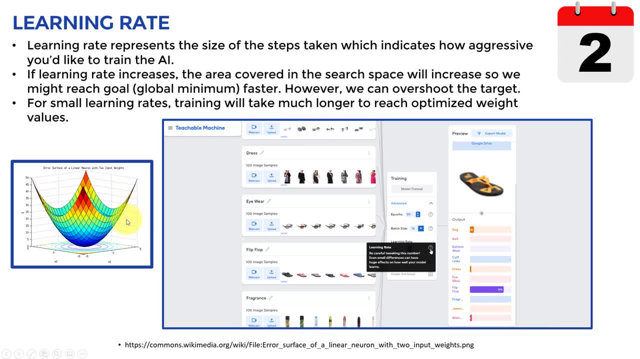 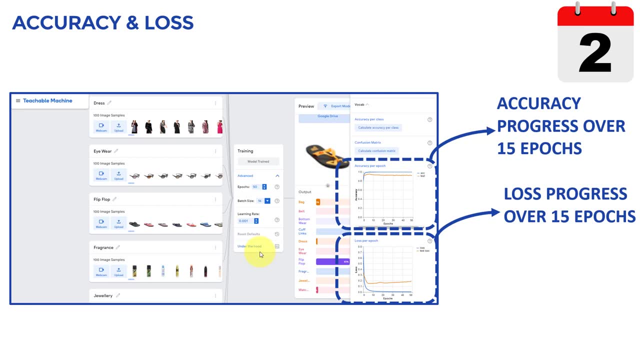 then training will take a much longer time for it to reach that point, but you are not going to be overshooting that target. okay, all right, so that simply concludes our learning rate, and then the last definition that i wanted to cover for you guys is accuracy and loss. so if you actually 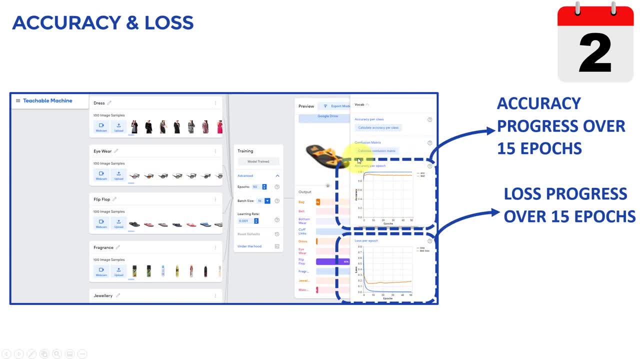 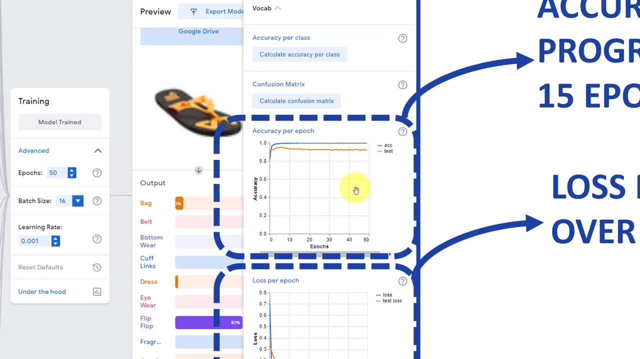 click on under the hood, you guys will see that here on the right hand side you will see graphs, and these graphs indicates the actual progress of our data, of our training over the number of epochs. so, for example, here i have the accuracy. so initially the accuracy wasn't too high, it was. 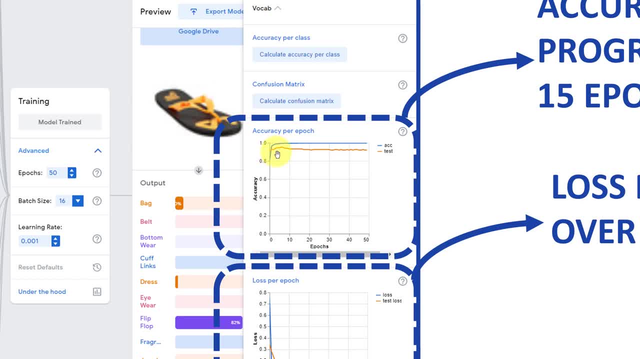 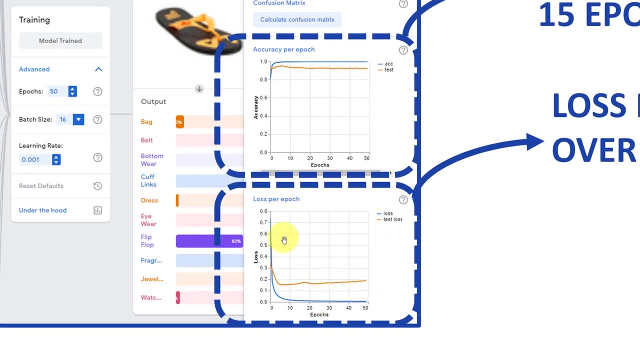 like 0.8 and then over time it starts to become better and better. now it becomes like 0.9, you know, and so on until it is almost 100. same deal as well for the loss, when you, when i say loss, think of it as more of an error. so the error starts very high. 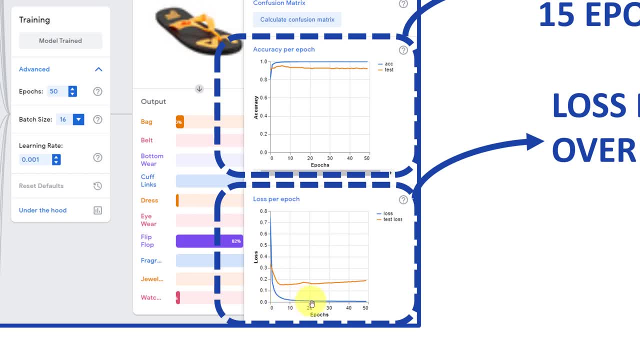 initially, and then over time, you guys will see that the error tends to go down, and please note that here i have essentially two types of accuracies and two types of losses too: one for the training set and one for the testing set, and what you guys see here is on the accuracy, on the 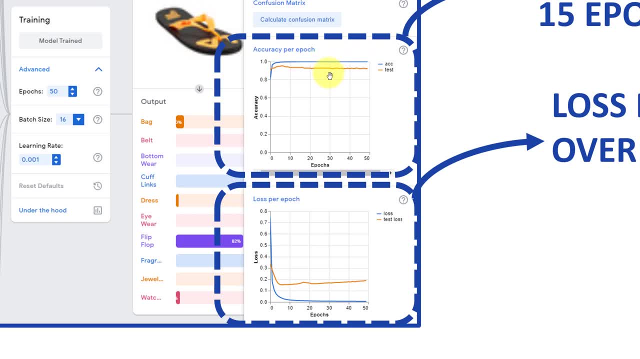 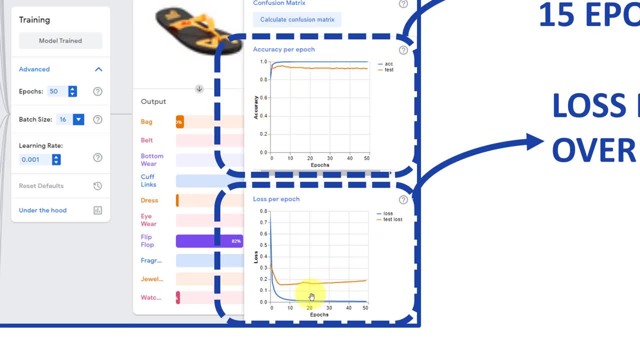 been seen by the model during training. and same deal as well for the loss. you guys will see that the loss or the error on the training data, which is my blue line here, tend to be less compare or smaller compared to the test loss or the error on the um, on the testing data set. okay, all right. 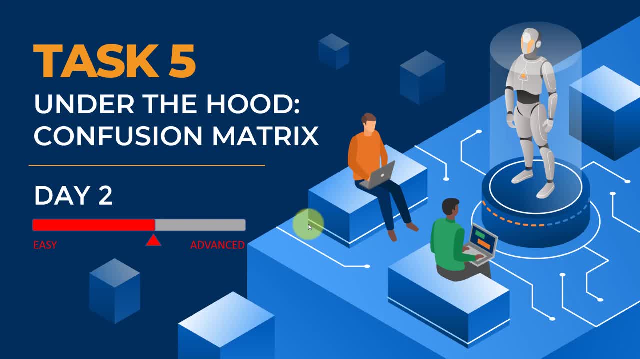 so that's it. that's simply all i have for task number four. i hope you guys enjoyed it. in task number five let's go ahead and cover a very important um definition, which is known as confusion matrix. please stay tuned, best of luck and i'll see you guys in the next task.